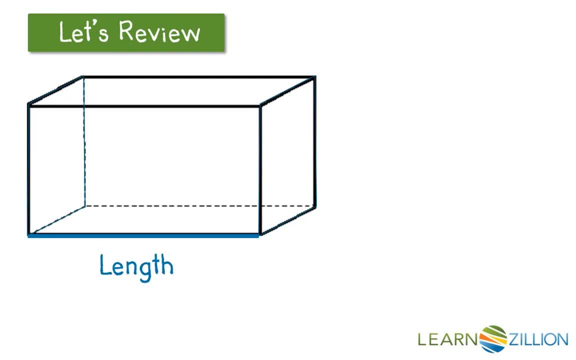 Another topic to review is the sides of a rectangular prism. So here we have the length, which is highlighted in blue, the width, which is highlighted in red and the height, which is highlighted in green, And there are congruent sides of the rectangular prism. 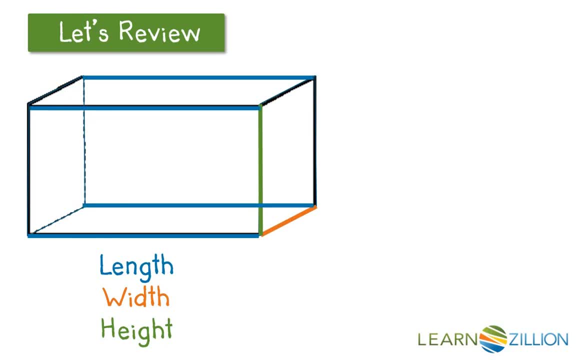 So here we have other equal lengths, equal widths and equal heights, And here we have a cube, And one side of the cube can be called the edge, And so all the edges of the cube are equal- A common mistake to make in these types of problems. 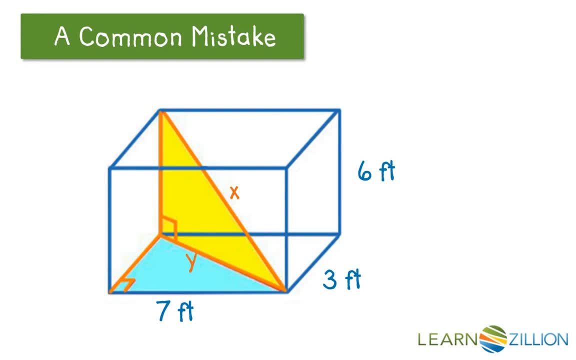 is not recognizing the two right triangles needed to solve the problem. So say, we're looking for the value of x in this problem. What sides of the triangle do we know? We only know the height of the prism is 6 feet. We still need to know what y is before we solve for x. 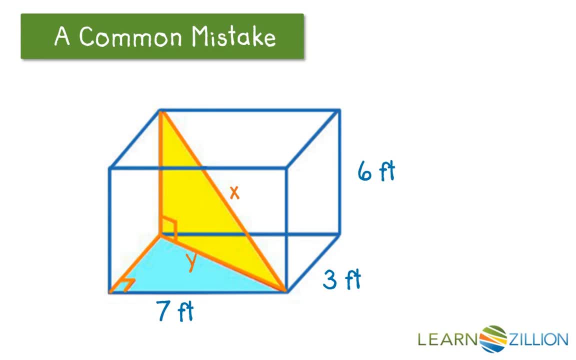 So one way to solve for y is to use the width and length of the rectangular prism, So in this case it would be 7 feet and 3 feet. Do not assume any side lengths when solving a problem of this type. So you definitely want to make sure that you recognize. 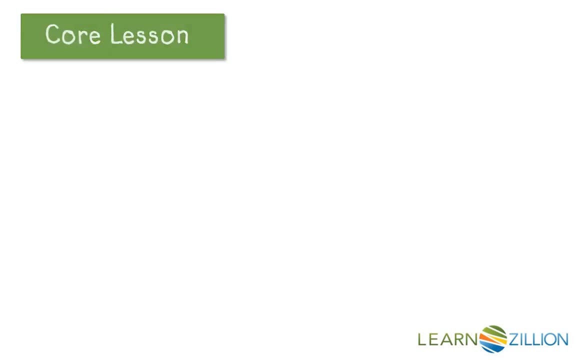 the two different triangles. So here we have a cube with an edge length of 5 inches. How can we find the length of the red line segment that is inside the cube If we draw a right triangle inside of the cube? so there's one side, there's the other side. 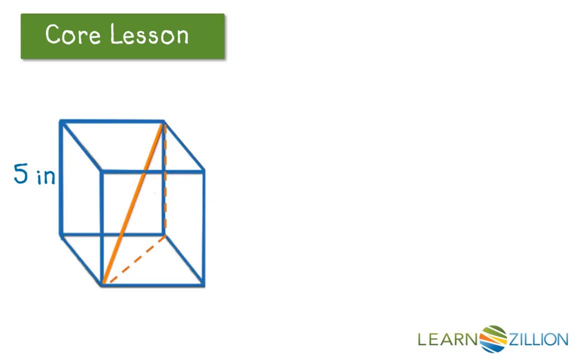 do we have enough side lengths to find the length of the red line segment? Well, right now we really only know that this side is 5 inches, So we're missing the bottom leg. in order to use the Pythagorean Theorem to solve this problem, 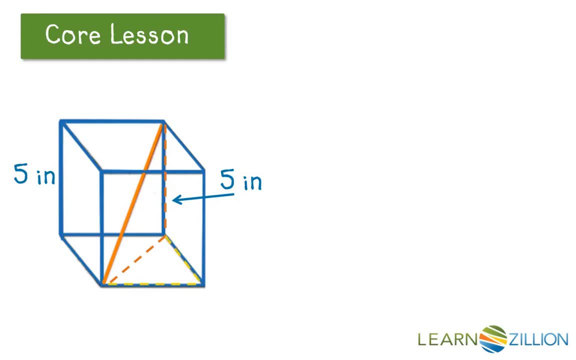 So let's draw another triangle. Here's one on the bottom. So we know that each of these sides of the triangle, or the legs, are 5 inches. So we can use the Pythagorean Theorem to find the bottom of our red triangle.